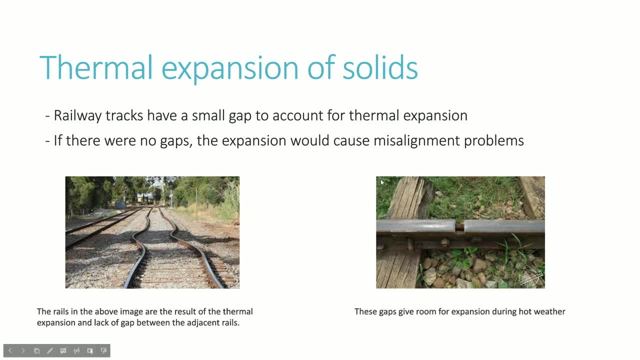 And so, for example, you can see on this right hand picture here that you have these tiny little gaps that are present on railway tracks, And this pretty much gives room for expansion when the weather does get very hot. And on the left hand side, this is what might happen if you don't put in the appropriate. 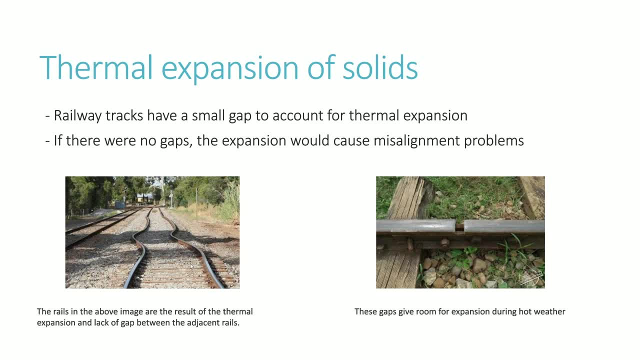 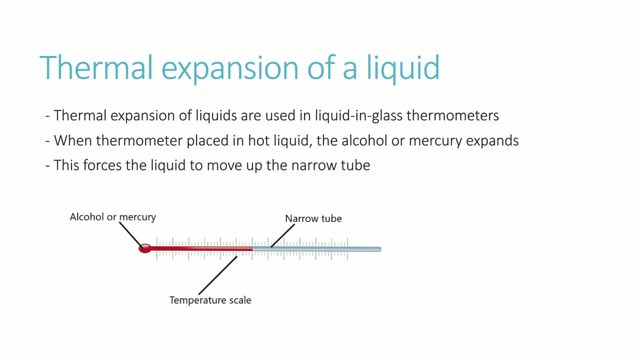 gaps to account for the expansion And you'll see that the thermal expansion has increased. It has pretty much just caused the track to become very misaligned and out of shape. You can also see the same thing in liquids: Thermal expansion of liquids. that property is used in liquid in-glass thermometers that. 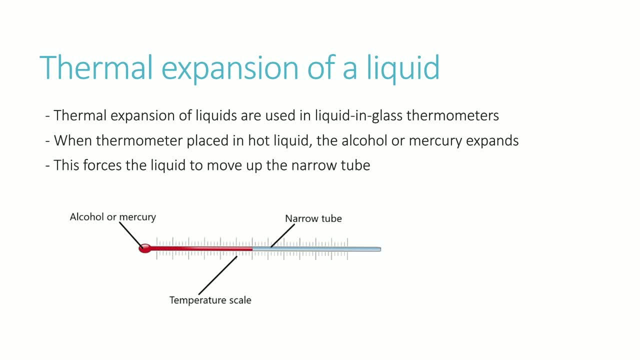 we'll be taking a look at in a bit more depth later on, And thermometers, of course, is a way to measure temperature and how that happens. is that the alcohol or the mercury that you put in the track is going to change The temperature that you put inside the narrow tube. will the alcohol or the mercury actually? 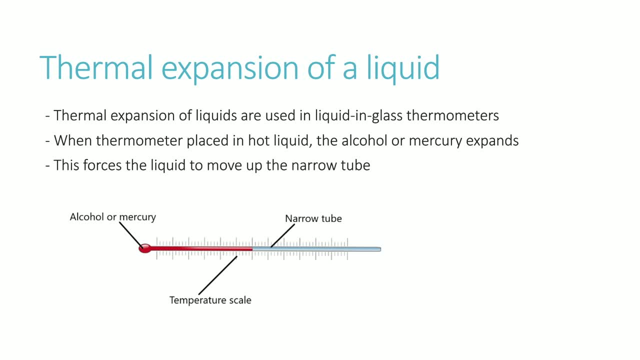 expand depending on the temperature. The higher the temperature, the more it will expand and as a result of that then you can use that property- an expansion- to measure the temperature of an object, And of course the cooler it gets, the less expansion and it sort of shrivels down and 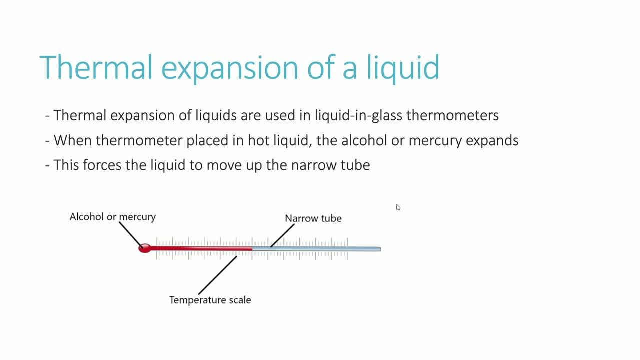 therefore it sort of goes towards the left hand side of the scale, So that thermal expansion of liquids is an important concept when we want to determine how we can experimentally determine temperatures of objects and the making of thermometers as a result. And finally, the thermal expansion of a gas. 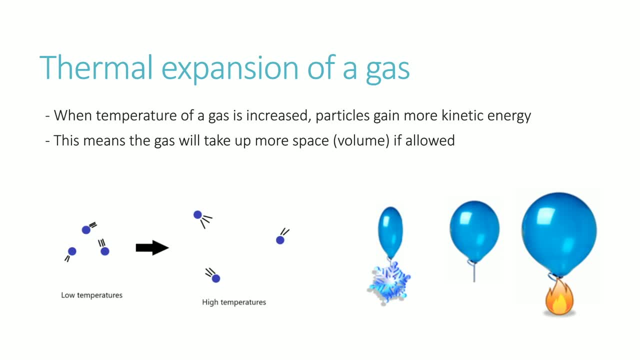 When the temperature of a gas increases again, particles gain increased kinetic energy And it will mean that the gas particles will occupy more space or volume. So it's going to be a very difficult experiment to do. that. That's all. Thanks for watching. 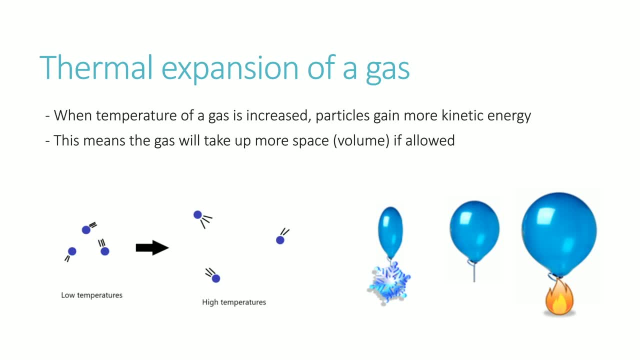 if it is allowed to do so, if it's allowed to become expanded. so that's a molecular concept here on the left hand side, as you can see the increased separation of the particles. but you know, if you take a look at the balloons here, you can clearly see that the volume of the balloons are different. of course, the 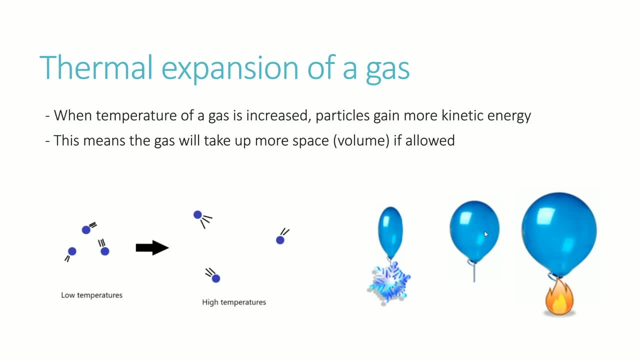 balloons themselves have a very stretchy wall allowing it to be expanded if possible, and very cool temperatures. the volume that the gas occupies is lower than in a higher temperature setting, where the gas particles will be more separated and you can see the increase in volume as a result of that. so let's 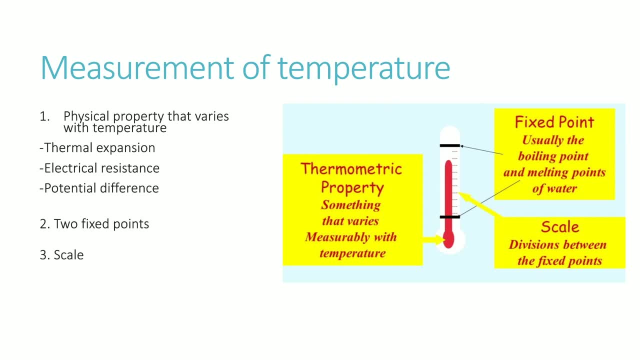 take a look at the concept of measurement of temperature, because we took a look at the fact that one important way that we can measure temperature is by using what we call thermal expansion- mostly, you know, alcohols and mercury's that you can find in glass thermometers. 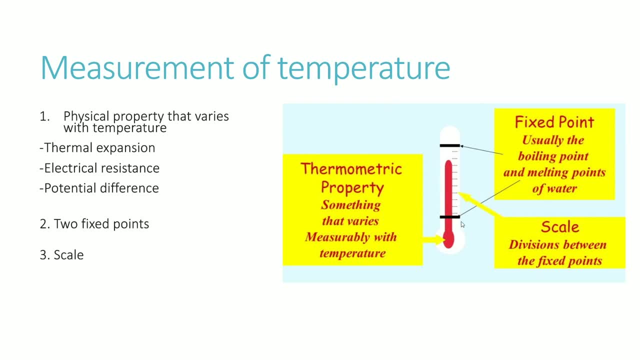 and how it works is: you've got a glass with a very narrow tube and inside of it you've got the alcohol or the mercury, and we're going to rely on the thermal expansion. that is basically something that varies measurably with temperature and, as we talked about, as the temperature goes up, then the expansion. 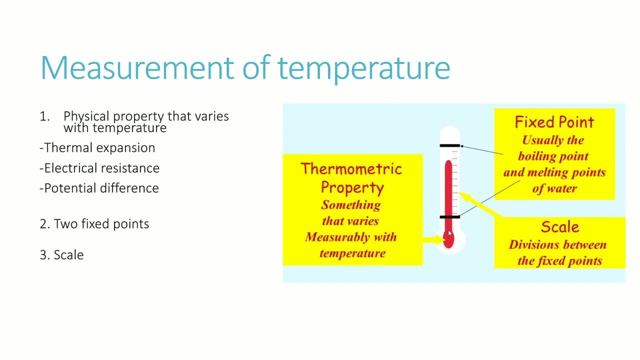 goes happy and as a result of that, the mercury or the alcohol will travel upwards the tube. Now this thermal expansion is just one type of a thermometric property, which is, you know, a property that varies with temperature measurably, and so thermal expansion is something that we can use, and of course we use that in. 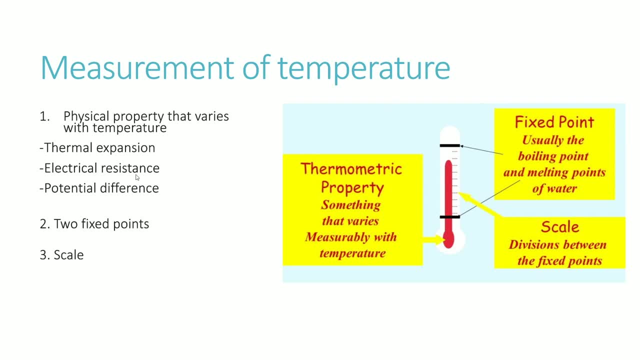 glass thermometers, but you can also use electrical resistance and potential differences, which is found in other types of thermometers and arguably more accurate ones than the in glass ones. but let's take a look at the in glass one for now. Not only do you need a thermometric property in this case, 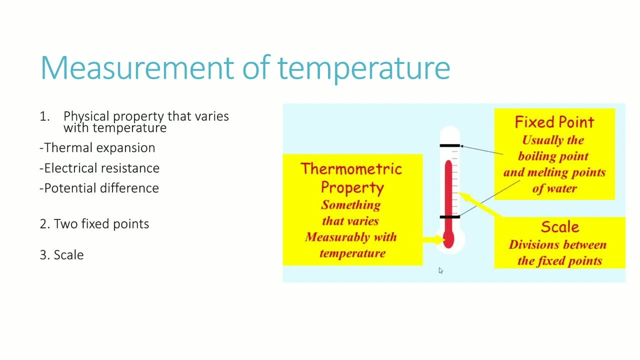 thermal expansion, but you need to figure out two fixed points that you can use for the scales, and so fixed points are important because it's it allows you to calibrate and make the thermometer consistent, like if you are. if you're making a device that can measure temperature of an object, then you need 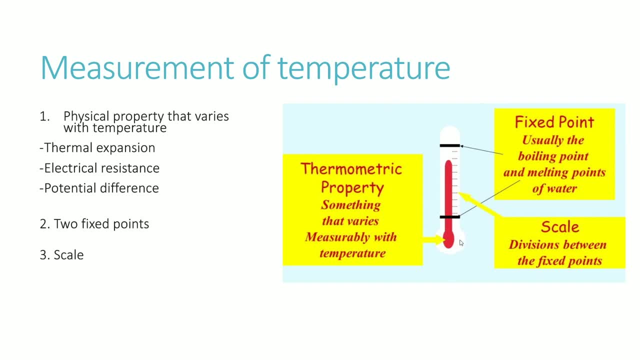 that to be consistent wherever you go like, if you measure the temperature with the thermometer here in New Zealand, let's say, of object A, and you measure another object in America with the same thermometer, then the thermometer needs to give you consistent readings, and one way that we can make the thermometer accurate and consistent is by using two. 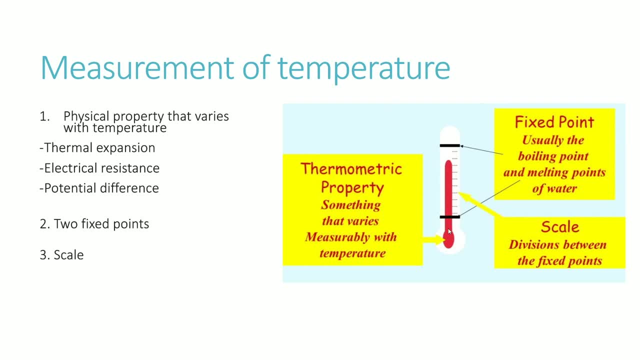 fixed points, which is the lower and upper end of the scale of the, the temperature measurement. Choosing the fixed points is something that is universally consistent, and you know universal consistency would be something like some sort of physical phenomenon that occurs at strict temperatures. the temperature itself can be arbitrary, it doesn't. 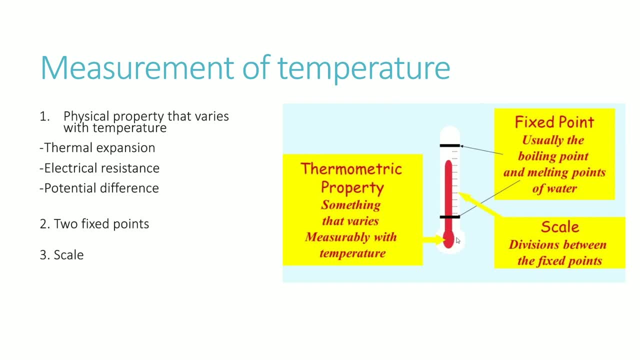 matter, but a certain temperature at which something is bound to manifest, and one good point would be the freezing point and the boiling point of water. no matter where you are in the world, water is always going to freeze and boil at the same temperature, and so, therefore, using those two things as the fixed points of a thermometer would be. 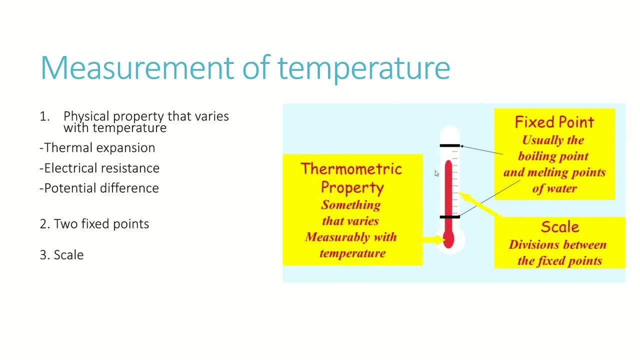 very helpful because then, no matter where you use the thermometer, then it's going to be scaled in proportion to the fixed points, which will be consistent no matter where you are. so the what, what happened with the Celsius scale is basically well, okay, well, the freezing point of water, we're going to call that. 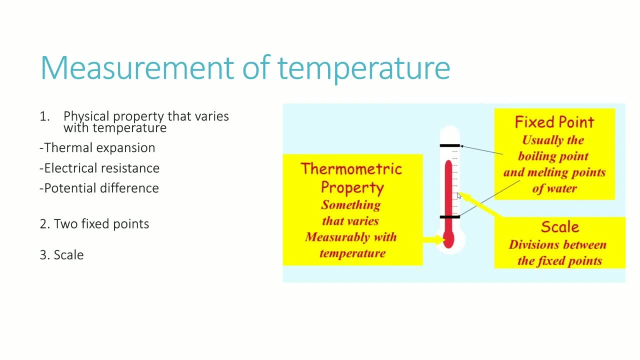 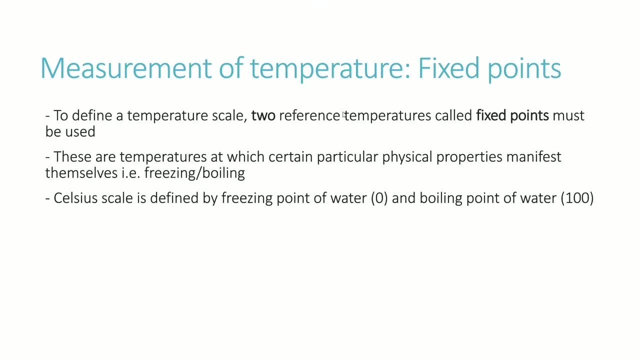 zero, and when water boils we're going to call that 100 and we're going to have even divisions of 100 going between those two realms, And that's pretty much your average thermometer. So here we're just talking a little bit more about the idea of a fixed point. 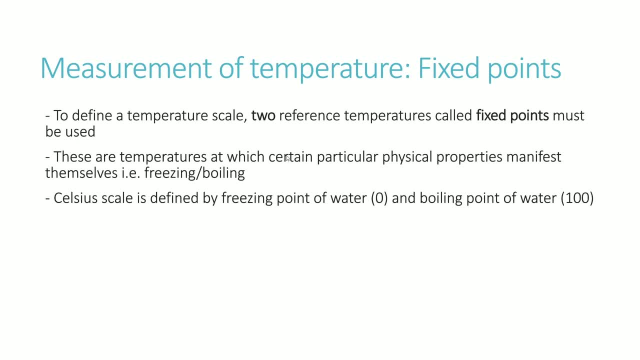 which can be sort of confusing in the beginning. but, as I said before, to define a temperature scale you need two reference temperatures, which are called fixed points, And most of the time we just use freezing and boiling points of water to determine these two fixed points because again, that's a universal temperature. 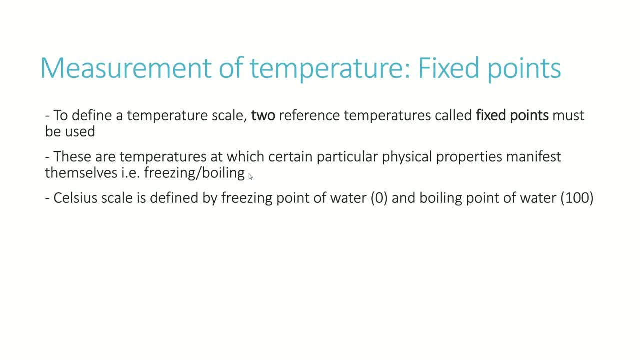 that exists throughout the world, And so we've got the freezing point of water being labelled as 0, and the boiling point of water as 100, and then you've got even distribution of scales of 100 units, going between the 0 and the 100. 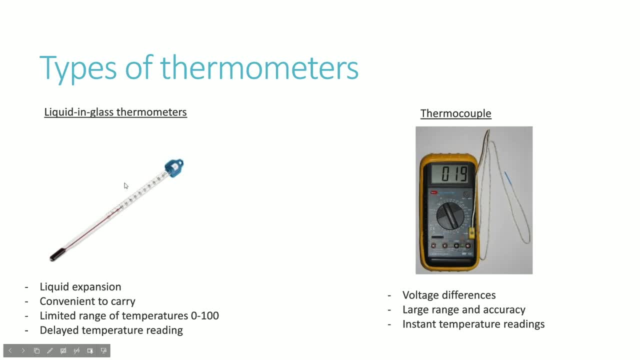 As I said before, you have different types of thermometers. The liquid and glass thermometer is using the thermal expansion to account for temperature measurement, so it relies on liquid expansion. It's portable, but it does have some limitations, especially when it can only measure temperatures between 0 to 100.. 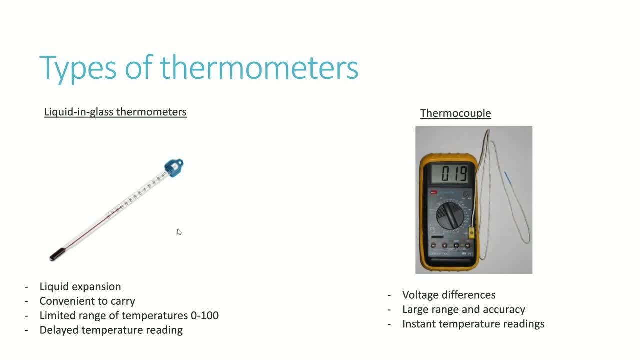 And also, if you've used one of these before, then you know that it takes a while for the liquid to sort of creep up and give you that measurement, so there's some delay in the temperature readings. A thermocouple is a different type of thermometer. 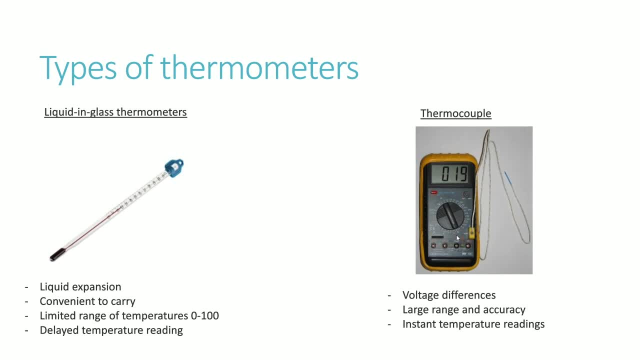 that you typically use to measure temperature. Thermocouple is a different type of thermometer that you typically use to measure temperature. It specialises not the expansion of liquids this time, but another thermometric property, which is voltage differences, The increase or decrease in temperature, or just measuring temperature in general. 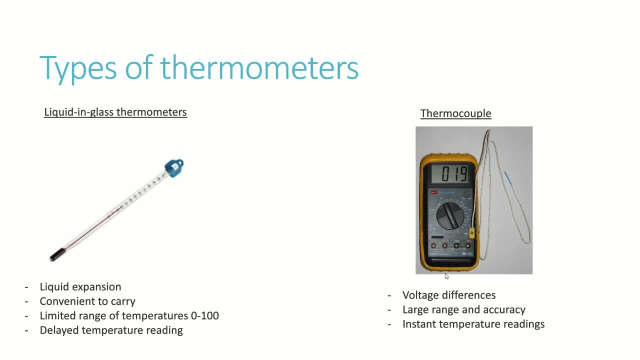 can be measured using voltage differences that you find between two different points, Because THAT actually changes evenly with temperature as well. But you don't have to dig too deep into that. ultimately is just using potential or voltage differences to calculate the temperature. 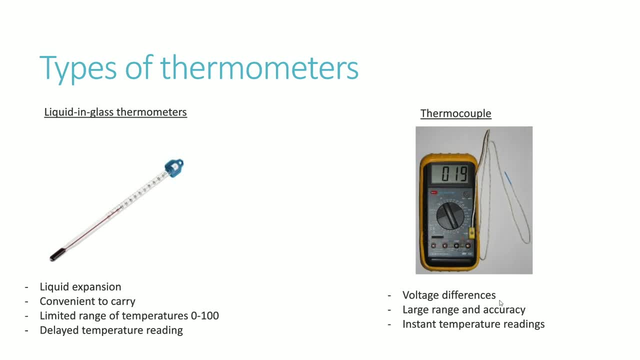 You get a much larger range of readings. It's not limited to just 0 to 100 degrees, so you can measure much more higher temperatures with this and with increasing accuracy, And the temperature readings are almost instant. You don't have to wait for the liquid to go up like you do in the liquid. 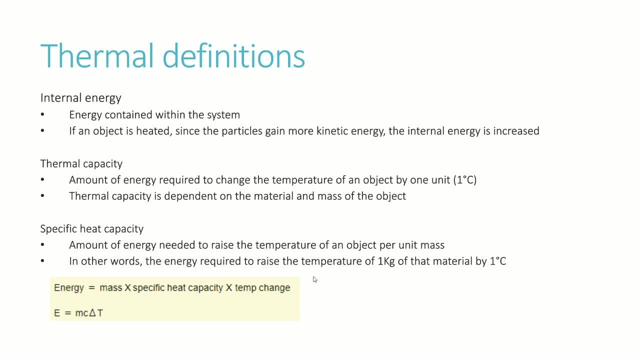 and glass thermometer. So this is where we get into some more complex stuff, which is not really that complex but requires some calculations on your end and things like that in exam questions, But ultimately you've got some important definitions that we have to look at. So the internal energy is the energy combined or contained within the system. 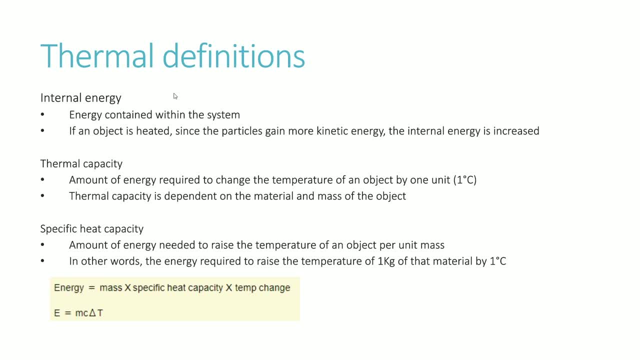 as a totality. As you increase the heat, or if you increase the temperature of an object by heating it, what that means is there's increased kinetic energy within the particles of that substance And inevitably that increases internal energy. So the internal energy is. 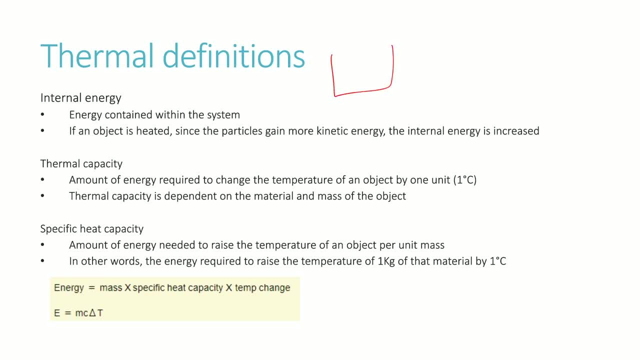 the total energy in a system. So if you increase the temperature of an object by heating it, what that means is there's increased kinetic energy within the system. And so if you have a box with particles, the particles will obviously have kinetic energy, but you've 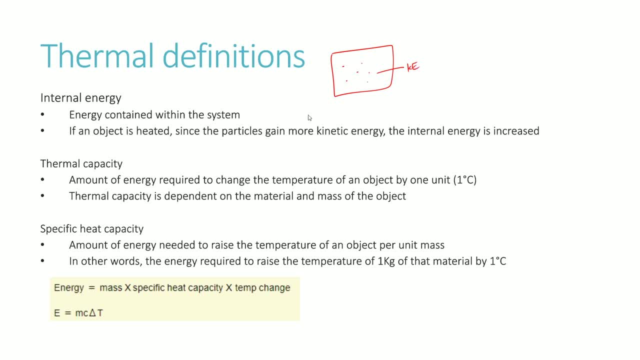 also got potential energies which are not kinetic, maybe between the bonds of the particles here. So you've got potential energies as well. And so ultimately, when you combine every single total energy within the system, you add that all up together. well that's. 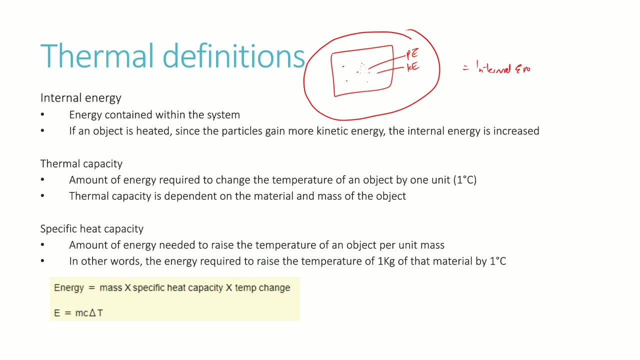 internal energy. So inevitably, as you heat an object, well its internal energy is going to rise because you're increasing the kinetic energy of the particles there. Thermal capacity is the amount of energy required to change the temperature of an object by one unit or one degree Celsius. 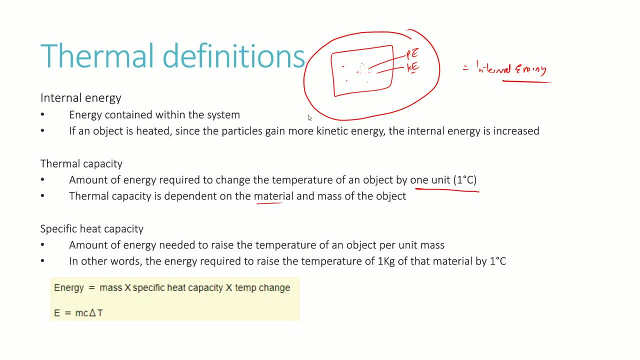 And the thermal capacity is dependent on what exactly material you're dealing with, because some materials will be more prone to increasing temperatures than others, and the mass of an object as well. Obviously, the bigger the mass, the more energy you're going to be able to generate, And so 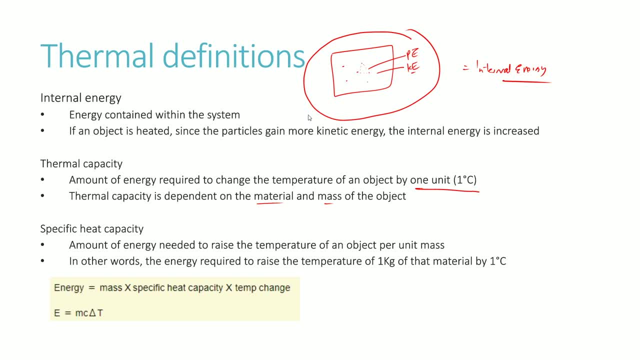 that's the more it's going to take to raise the temperature of the object. So thermal capacity is basically just when you've got an object, you want to figure out how much energy it takes to raise the temperature by one degree Celsius. So if it takes 1,000, 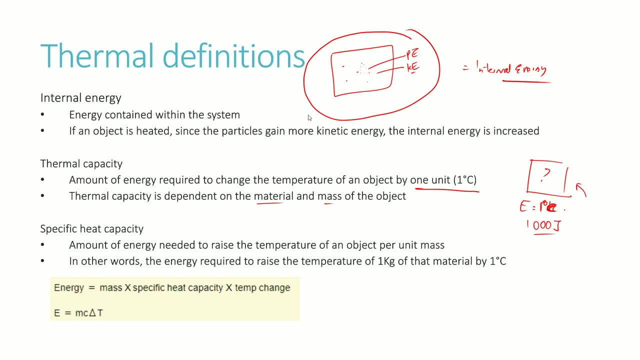 joules of energy to raise this object by one degree Celsius. well, there you go. That's the thermal capacity. Now the difference between thermal capacity and specific heat capacity is this time: with specific heat capacity, it's the amount of energy that you need to raise the temperature. 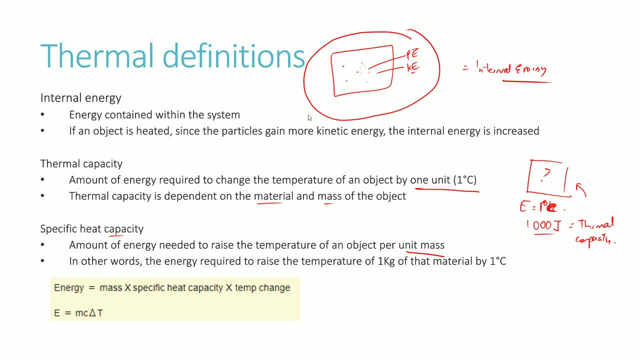 of an object per unit mass, In other words the energy required to raise the temperature of one kg of that particular material or substance by one degree. So you can see how there's a difference between what the thermal capacity is. It doesn't matter what the mass is. how much does it take to? 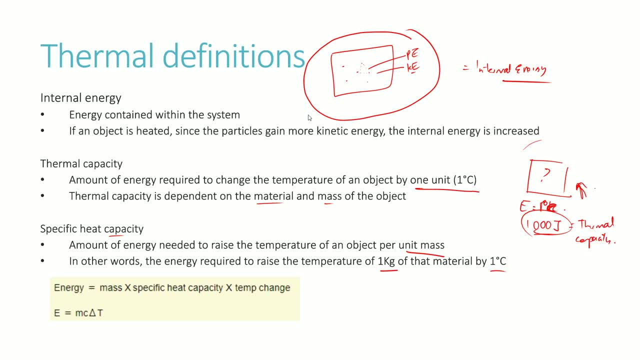 raise the temperature of this entire object by a certain degree Celsius, or even 10,000 entire object by one degree Celsius, but specifically heat capacity. you take into account the mass of the object and say: well, how much does it take to raise the temperature of one kg of? 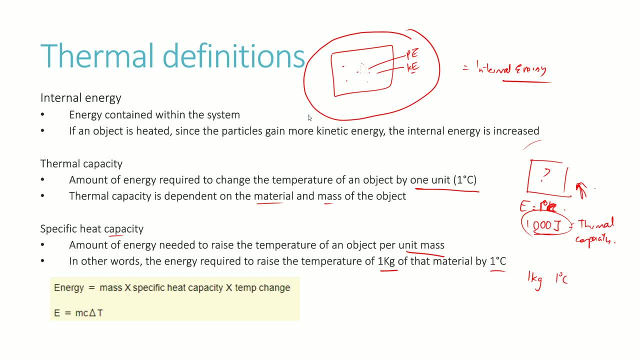 that material by one degree Celsius. So therefore, what it means is, if you have the thermal capacity of 1000 joules, then all you need to figure out the specific heat capacity of that object is simply the mass. For example, if the mass of this substance was 1000 kgs, then the specific heat capacity 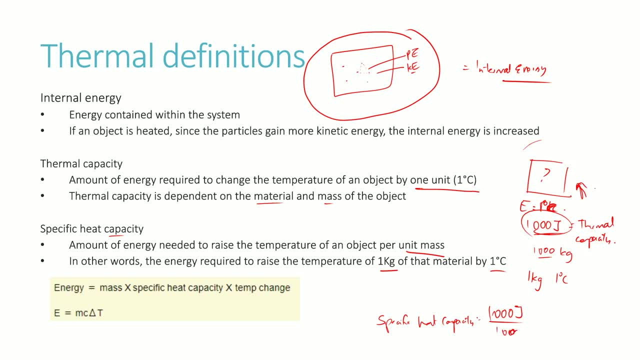 would be 1000 joules divided by 1000 kgs. So that will give you 1 joules per kg, I suppose. But if you take a look at the temperature of the object, you'll see that the mass of the object is 1000 kgs. 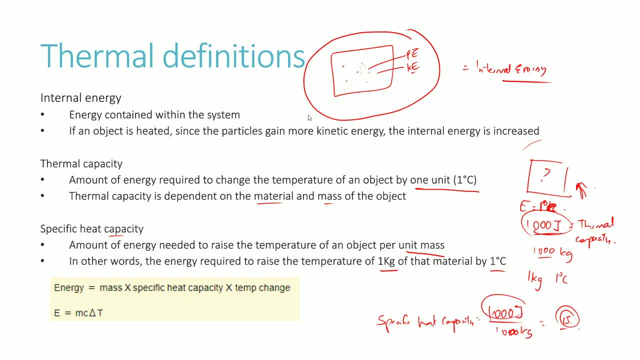 If you take a look at the concept here, it took us 1000 joules thermal capacity to raise the temperature of the entire block by one degree. and because, with specific heat capacity, we want to know how much it is per kg, well, all you have to do is divide that by the mass. 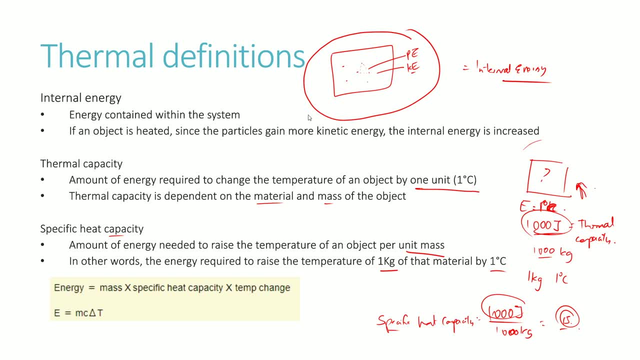 But ultimately speaking, generally the calculations that you'll do in your examinations, you don't really work from thermal capacity. The general formula that you'll be looking to use would be: energy equals mass equals mass, times the specific heat capacity times the change in temperature. 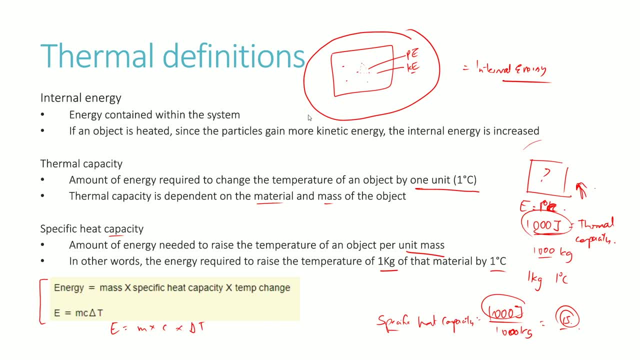 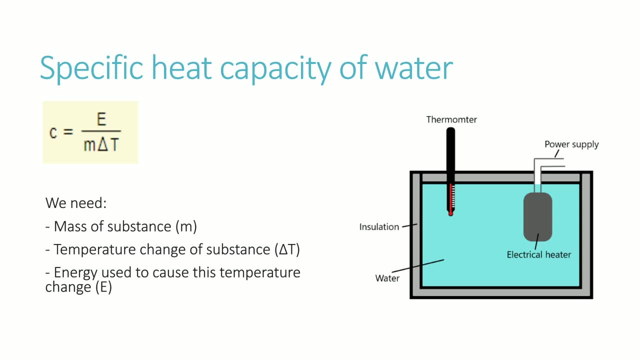 That's what the formula is and we'll be going through a few examples of that in a second. So this is just a rearrangement of the formula, because a lot of questions will be asking about actually determining the specific heat capacity of water and experimentally determining. 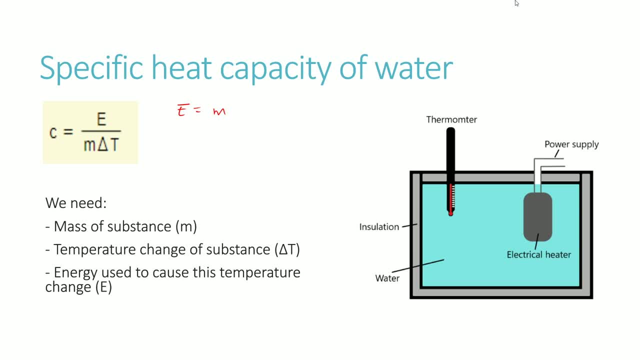 that. So the original formula was: E equals M times C times change in temperature. right, But you know, By rearranging the formula in order for us to figure out C, which is the specific heat capacity of a substance, in this case, let's experimentally determine water, then you've. 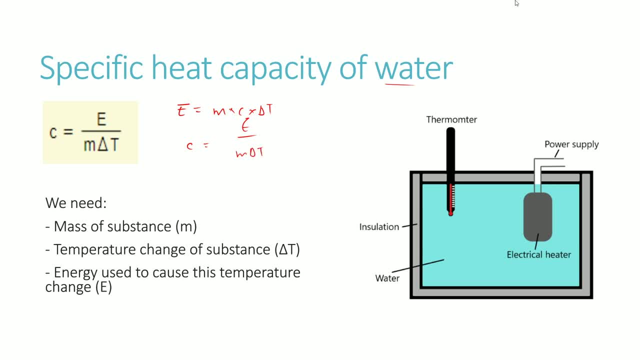 got E divided by M times the change in temperature, which is this formula. here, Mass is, of course, the mass of the substance. the temperature change is simply how much the temperature changed during the experiment, and the energy is the energy that we used in order to create this formula. 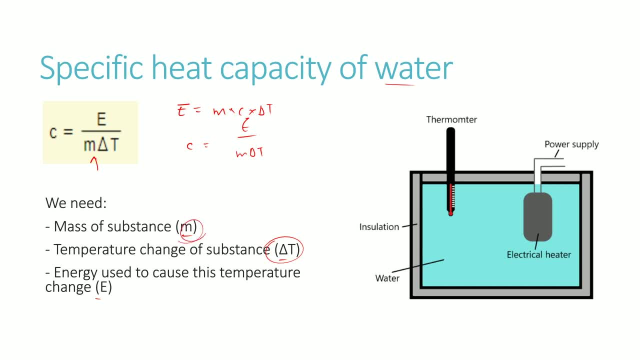 So we're going to use this equipment or this experimental set up. we're going to have a thermometer that's going to be able to measure the temperature of the liquid water that we're dealing with. The water will be present inside this insulated box that also has an electrical heater that 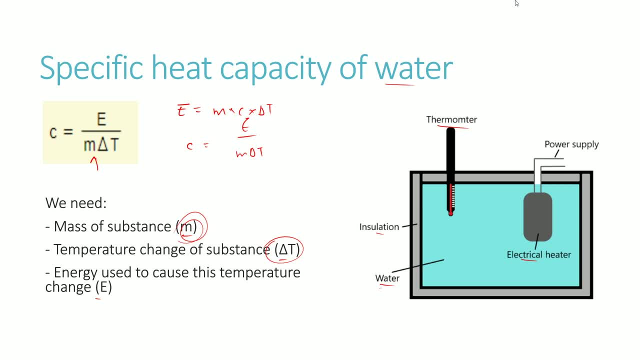 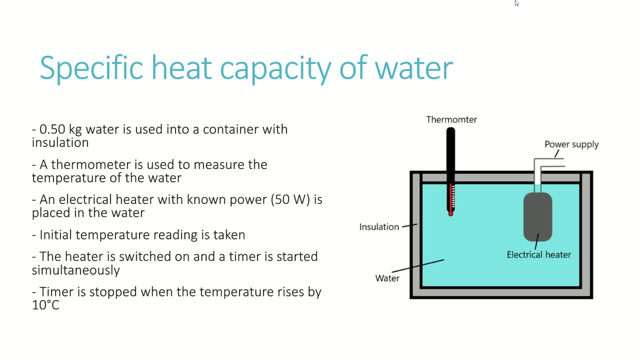 is going to start to gradually heat up the water. So Just imagine that the mass of the water that we're using here is 0.5 kg and we put it into this container that's insulated, that's got a thermometer that can measure the temperature. 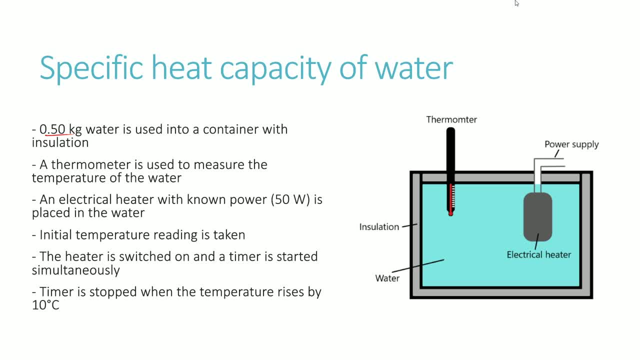 and also the electrical heater that's going to start to heat up the liquid. The thermometer is going to be used to measure the temperature, as I said before, and the electrical heater is going to heat up the liquid and it's going to have a known power. 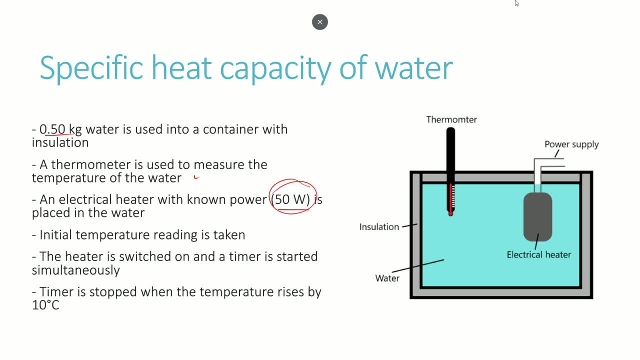 of 50 watts, and this value is important because that's v. 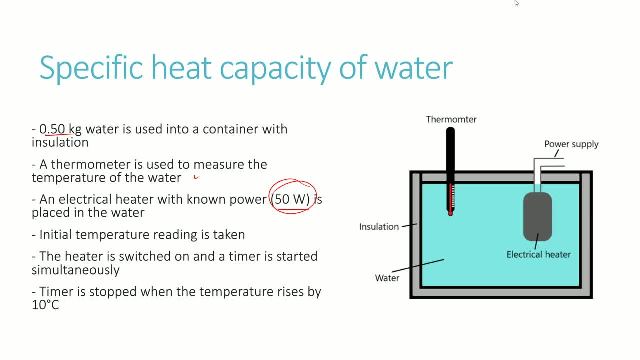 vGAW determine the energy, So initial temperature reading is taken. Whatever the temperature is, you start with that initial temperature being a certain amount And, of course, the idea is to figure out the final temperature as well, which will occur after a certain amount. 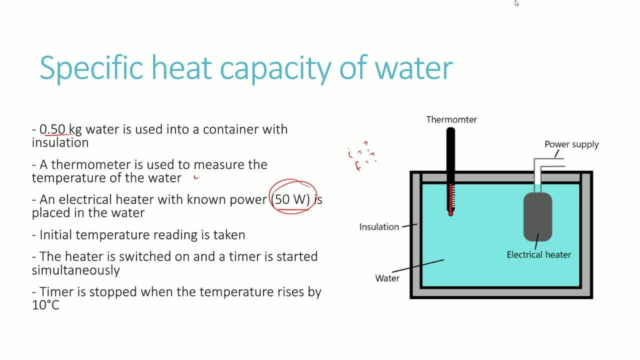 of time has passed, So the heater is switched on and you start the timer simultaneously. So this is 50 watts, by the way, And so, basically, you wait for the electrical heater to start heating up the liquid and you take a look at the thermometer and you wait for it to. 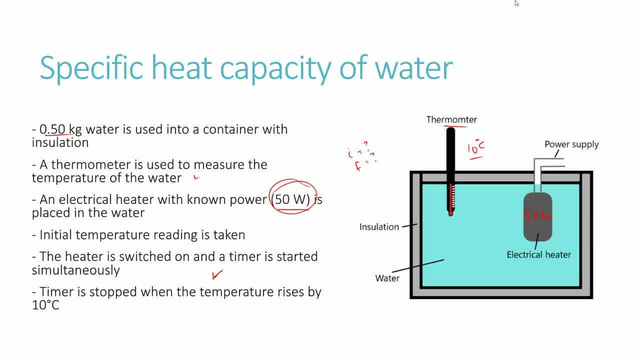 reach an increase in temperature of 10 degrees Celsius, And so what we know, then, is that the change in temperature is 10 degrees Celsius, Because no matter what temperature you start off with- room temperature, let's just say, is like 25 degrees- then you wait for the 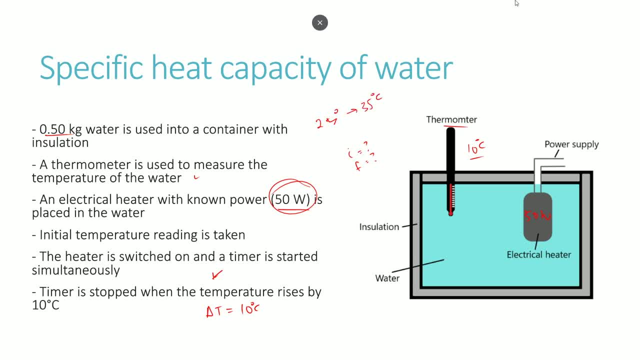 temperature to increase by 10 degrees, which is 30 degrees, Maybe 5 degrees, but ultimately the temperature change is always going to be 10 degrees celsius, because that is what we determined it to be. You could have waited for like 20 degrees. 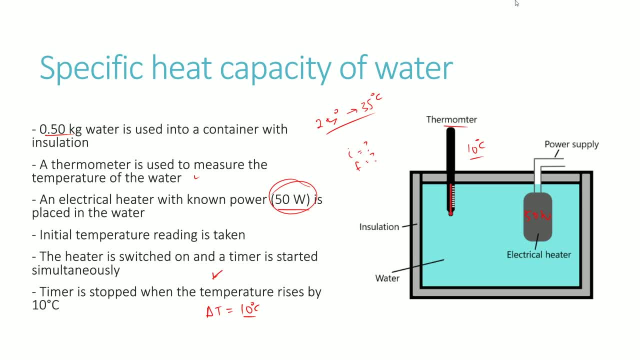 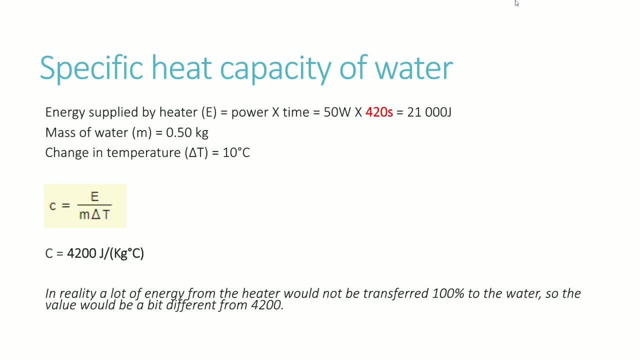 increase in temperature or 5 degrees increase in temperature, It doesn't matter, but ultimately the change in temperature is what we are looking at. So in order for us to determine the heat capacity or the specific heat capacity of the water, then we need to figure out how much energy we supply the system in order to create that. 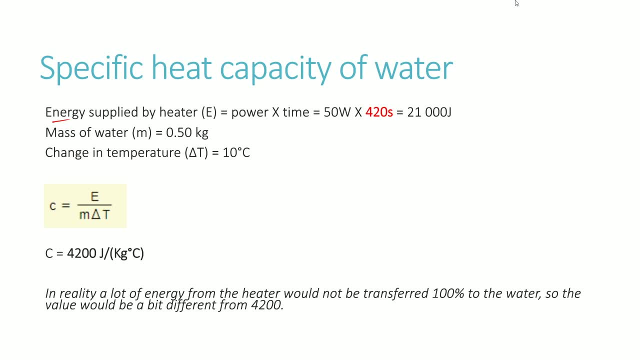 10 degree temperature change. And remember, energy is power times time. so 50 watts times 420 seconds, which is assuming that you would have actually experimentally determined that, because, remember, you started off timing as soon as you turned on the heater and then you're stopping the time and stopping the heater when the temperature rises 10 degrees. 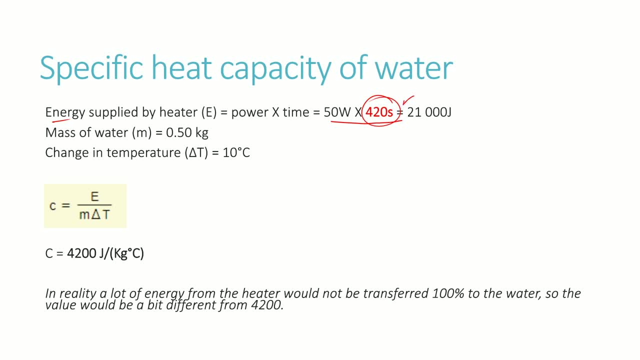 And we're just going to assume that the time it took was 420 seconds, Then what you get is a total energy of 21,000 joules, The mass of water, as I said, was 50.5 kilograms and the change in temperature is 10 degrees. 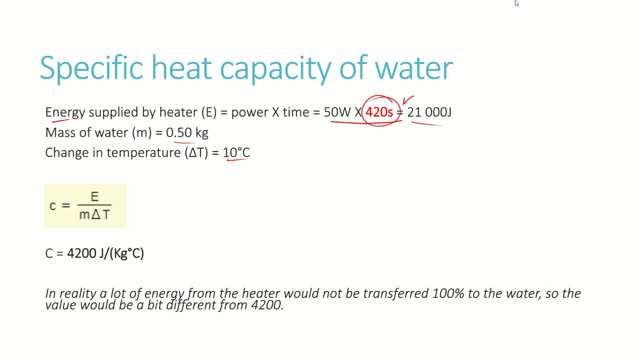 If you put that into the formula of 21,000, divide that by mass times the temperature change, Then you get 4,200 joules per kg degrees Celsius, And so in reality a lot of the energy from the heater would not be 100% transferred, so the value that you might get in the real world might actually be different from 4,200. 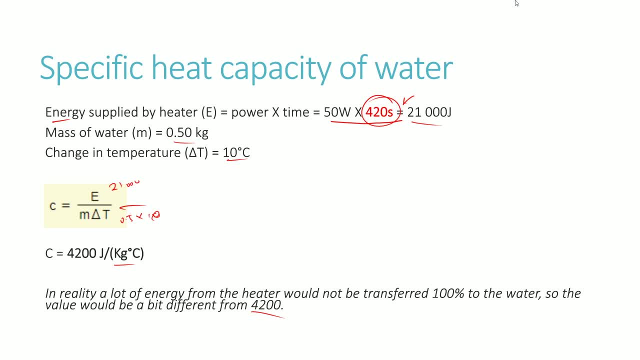 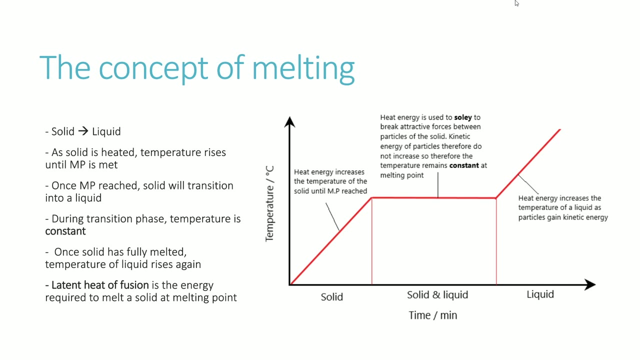 But ultimately speaking, with the assumptions that we've gone through here, that's the value that we get, So hopefully that gives you an understanding of how this formula is used in this particular experiment. So let's take a look at the concept of melting. Remember, we talked about the fact that the states of matter can change from a solid to liquid to gas. 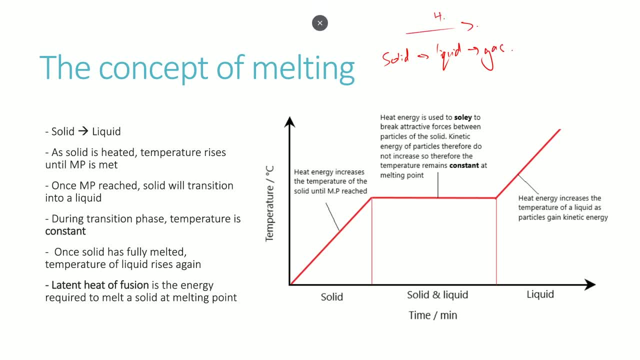 And we do that by heating—by giving molecules kinetic energy for it to separate amongst from each other. Of course, by cooling down you're achieving both normal and intermittent radiation execution of the molecules. For this reason, this process is also known asそうそう 수정. And we do that by heating—by giving molecules kinetic energy for it to separate amongst from each other, of course by cooling down—enough about 5 kg. And when you do this, you're measuring exactly where this potential will be. 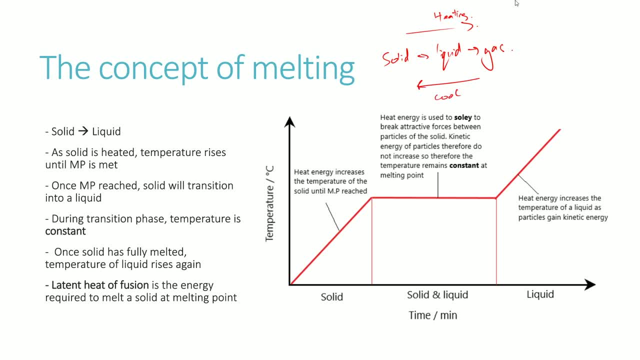 Notice that if you're using a sort of liquid, you'll get some like in quantum Имillah, a fraction thatение, because we will have a fraction that can multiply to green to make zero. you achieve the reverse process, and so if you take a look at a graph that maps temperature and the 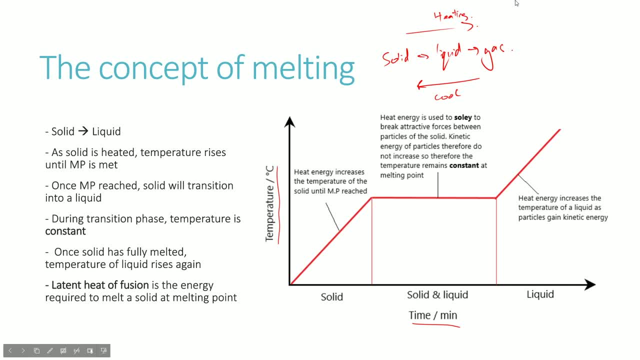 time, then you'll come to find something fairly interesting. so, as a solid is heated, the temperature begins to rise, and that makes sense, because as you increase the heat energy, you increase the temperature, which means that the kinetic molecule, kinetic energy of the particles are getting higher, and so that that all makes sense. what's interesting, though, is when you reach the melting. 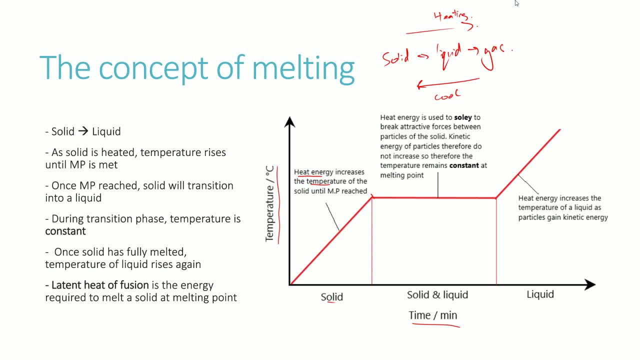 point now. melting point is the point, the degrees at which the solid begins to change into a liquid. you'll start to notice that here on the graph during the time that the solid and the liquid is sort of together, which is the transition period. right, this is the period between where the solid becomes a liquid but it hasn't fully turned into a liquid. 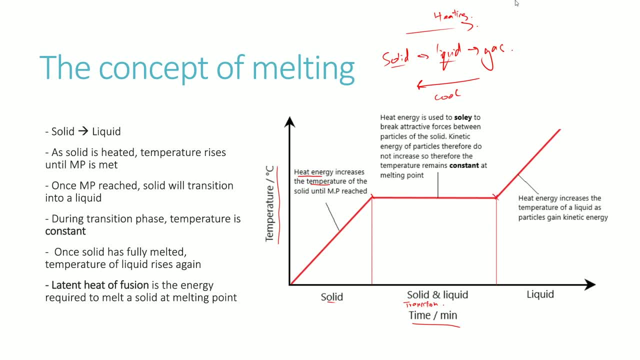 during this period, the temperature change is non-existent, the temperature is stable, which is, which is interesting, um, because you know you're still heating the substance. but why is the temperature not increasing? why are the kinetic energies of the particles, or the average kinetic energies, i should say, of the particles, within this transition state? why is it not increasing? 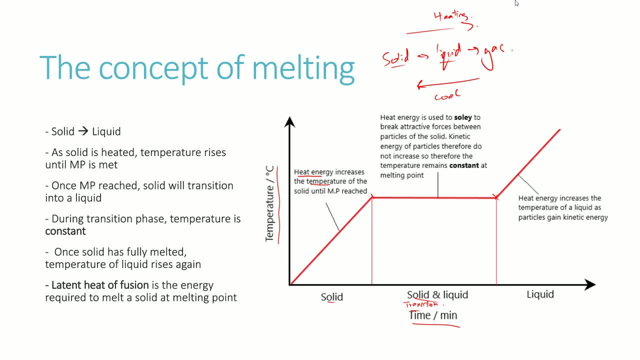 and so the reason for that is because the heat energy during this transition phase is not actually used to increase the kinetic energy of particles. okay, and remember, the kinetic energy of the particles is what causes increase in temperature- but instead the energy that you use during this transition period is used only to 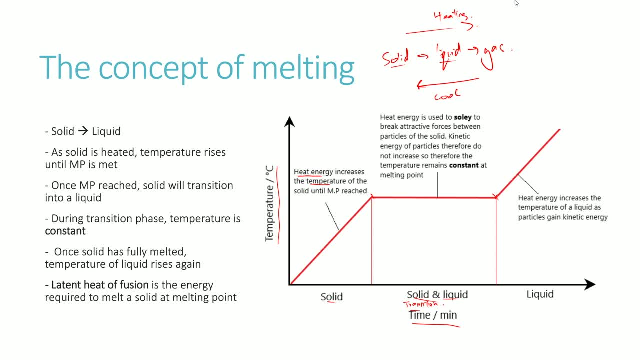 break attractive forces between particles within the solid- remember, solid- particles are very close by together, and so when you are transitioning from a solid to liquid, what it really means is that the particles are becoming more spread out apart. you have increased separation. so what i'm going to do is i'm going to use the heat energy that's being used to increase the kinetic energy. 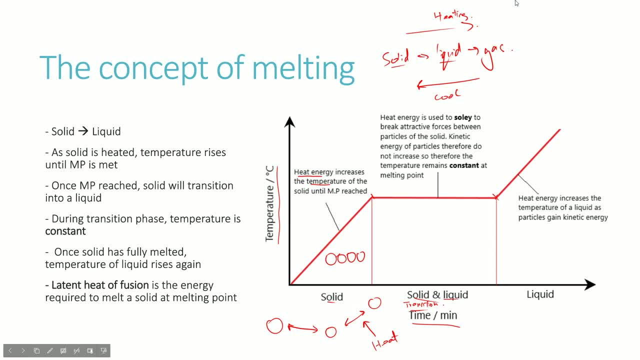 of the particles, and what that means is that during this transition phase, the heat that you're inputting into the system, you're not using that heat to increase the kinetic energy of the particles. the kinetic energy of the particles stay exactly the same, but what you are doing with that heat is 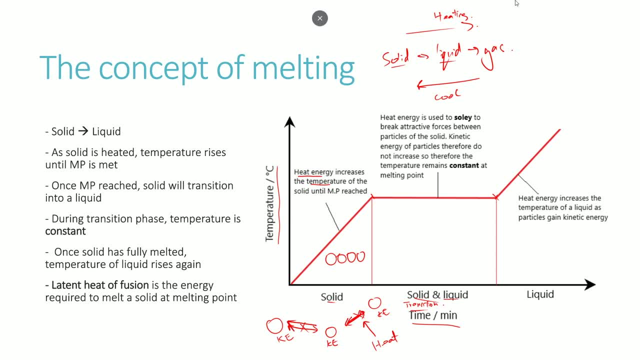 you're breaking apart the bonds between the particles and making it more spread apart from each other. okay, and so that's where the energy is going, and, as a result of that, the kinetic energy of the particles is going to increase in temperature, and that's why the temperature remains constant. 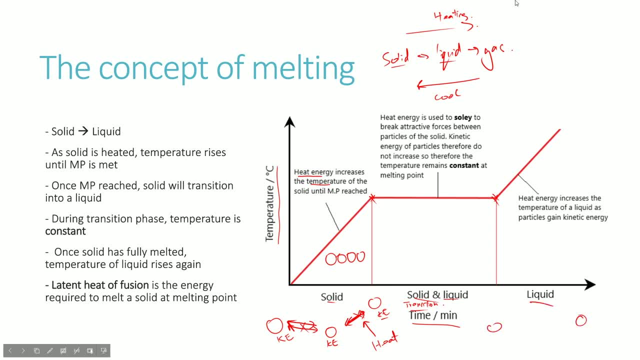 throughout this transition phase. once the liquid has fully formed, then you've got your standard liquid. and again when you put in the heat energy, then the heat energy is going to be used to increase the kinetic energy of the particles. and as the kinetic energy of the particles become, 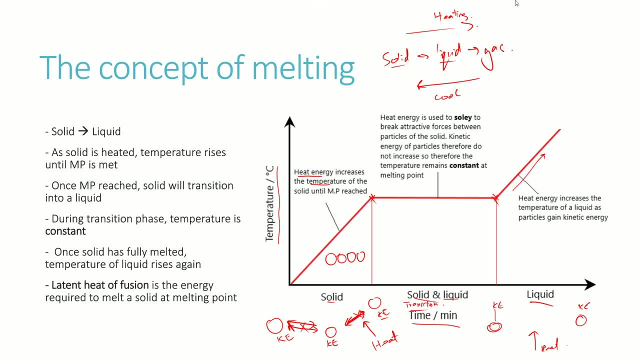 raised, then so does the temperature, by definition, and you can see this graph heading upwards again. after that transition phase is over, energy that is required for you to fully transition the solid to liquid. We're talking about this phase here. You can see that the energy isn't used to increase the temperature, but ultimately, 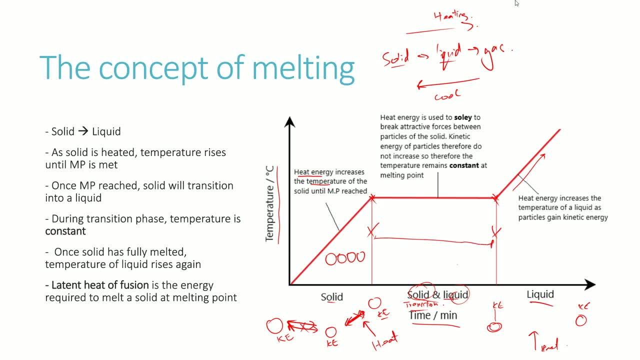 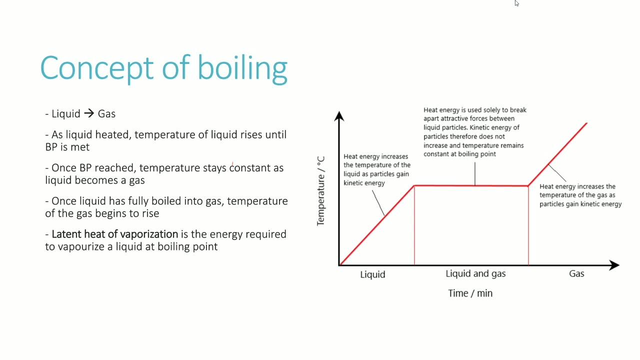 that same energy is called the latent heat of fusion, which is basically the energy that is required to melt a solid at its melting point. You can say the same thing about the transition between a liquid to gas. As the liquid is heated, the temperature of the liquid begins to raise, which is here. You can see that. 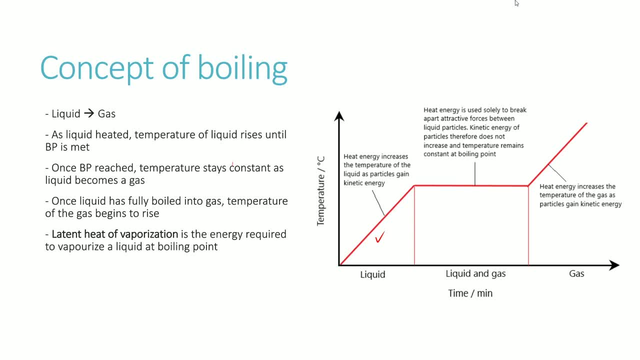 the temperature rises as you heat up the liquid, but once the boiling point is reached, the point at which it starts to become a gas, then what you'll find is the temperature increase stabilises and you don't get any increase in the temperature of the substance during. 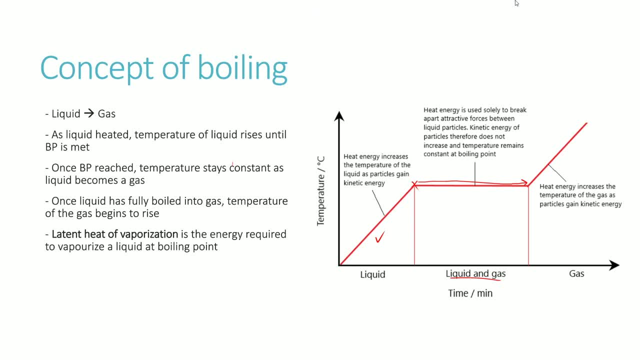 the transition phase between liquid to gas. Just to go through that one more time again: the liquid particles are like this, and the heat energy that you use in the transition phase between liquid and gas is used to break apart the bonds that exist between these two particles and cause that separation. That's. 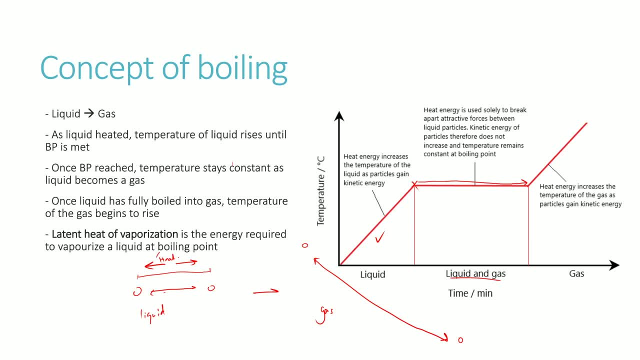 what you're using. That's what the heat is doing. The heat is using in this case is it's using the heat that is being put into the liquid to make the bond, and a bond is using, in this case, the heat that's being put into the liquid. 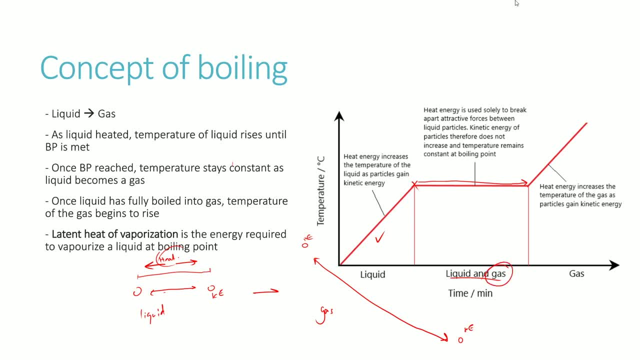 to make the bond and if it does, then essentially the temperature doesn't increase. The temperature is going to stay exactly the same until the gas is fully formed. then the increase in temperature will result due to the increase in kinetic energy that is being 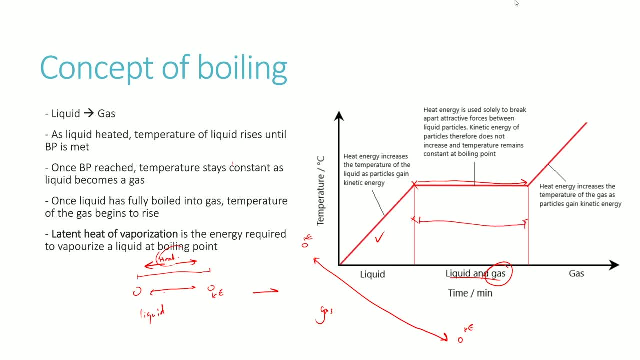 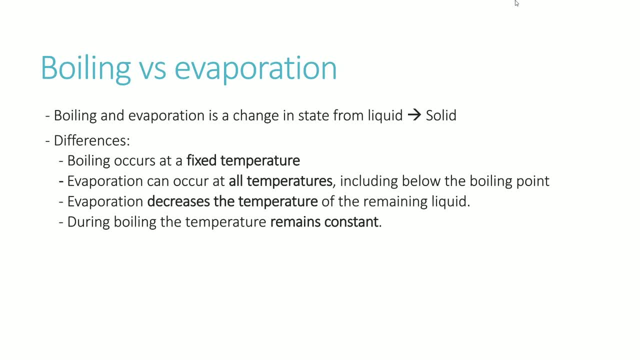 the substance. Remember, boiling and evaporation are very different. Boiling is basically, it occurs at a fixed temperature, So all substances will have a certain temperature at which the heat is enough to start to break apart the bonds, And so boiling will always occur at a fixed temperature, whereas evaporation can happen. 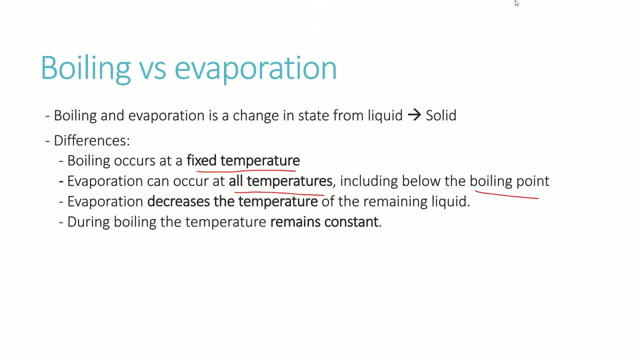 at any temperature, including below the boiling point, And that makes sense. Remember when we talked about evaporation. if you're still a bit confused about that, I'd recommend you go back and see my previous video. We go through evaporation in a bit more detail there. 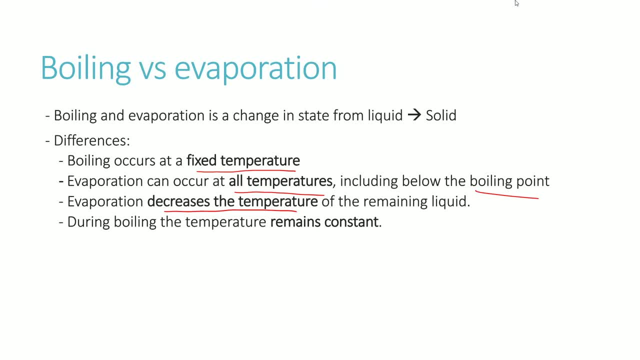 Evaporation decreases the temperature of the remaining liquid, whereas in boiling, as we took a look at the graph before, it's going to. So if this is, If this is liquid during the transition phase between liquid gas, then the temperature 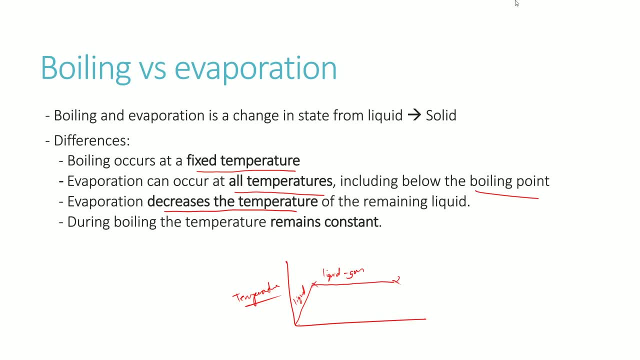 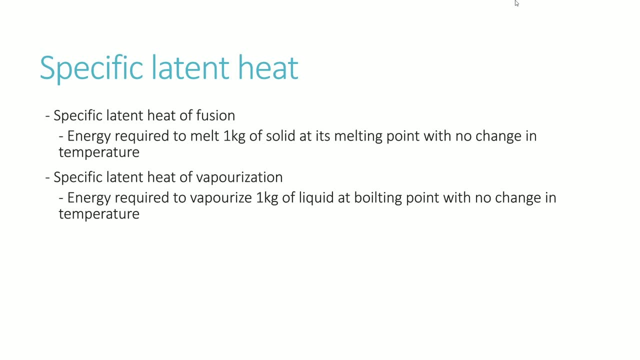 stays constant. So that's one other very important difference between boiling and evaporation. So let's take a look at specific latent heat, because that's the heat that we took a look at during that transition phase from whether it's liquid to gas. 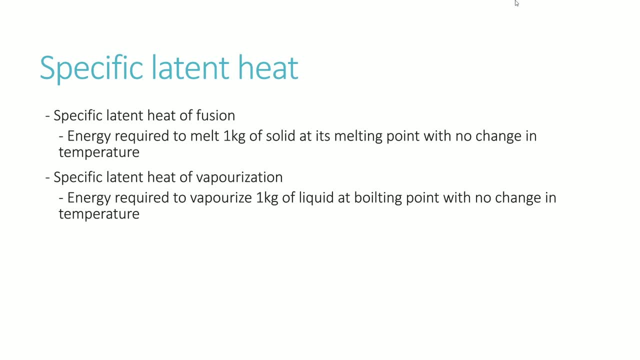 Which is latent heat of vaporization, or the transition from solid to liquid, which is the latent heat of fusion, And so that's latent heat, but specific latent heat. So, as we looked at before, with specific heat capacity, you integrate mass into the equation. 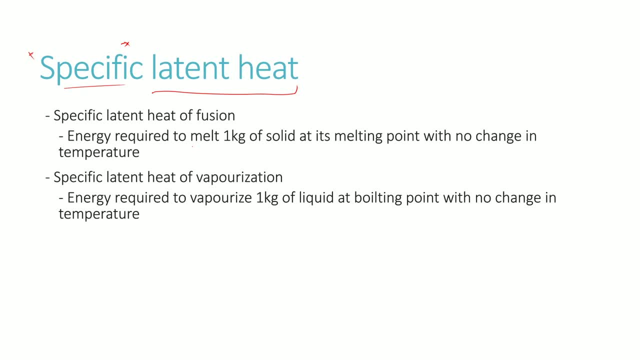 So the specific latent heat of fusion is the energy required to melt 1 kg of solid at its melting point with no change in temperature. And so we're specifically looking at the segment of the graph where it goes like that. This is what we're looking at. 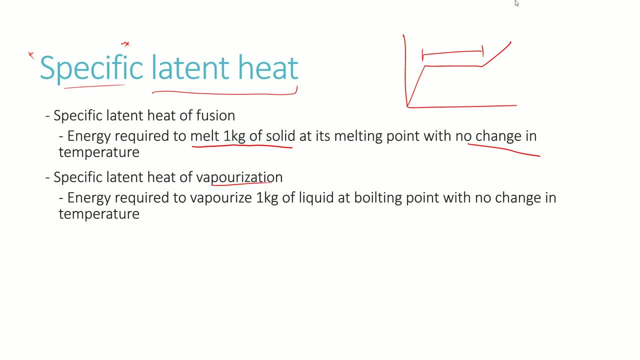 And so the specific latent heat of vaporization is the same thing, except for the fact that it's the energy required to vaporize 1 kg of solid. That's the latent heat of fusion of liquid at boiling point, with no change in temperature. 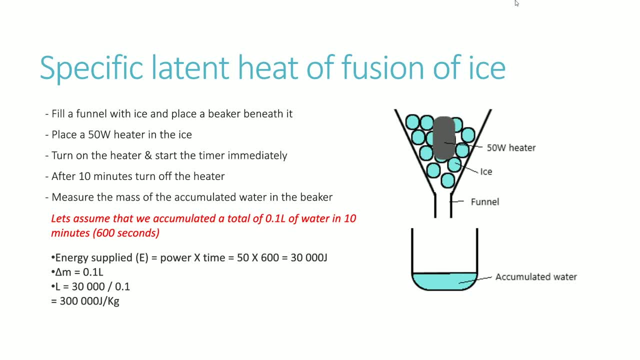 So the specific latent heat of fusion of ice can be determined by this experimental setup where you've got a funnel with a few blocks of ice and you've got that 5 watt heater there again. and the watts are important because that allows you to calculate the energy that 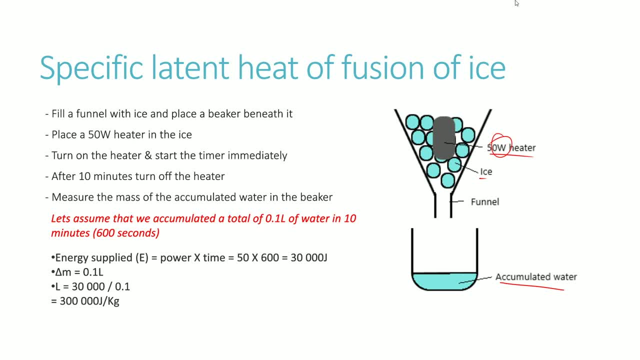 you're putting in and you've got the water that becomes accumulated underneath the funnel with a beaker. So you're going to fill the funnel with ice and place a beaker beneath it. with a 550 watt heater, You're going to turn on the heater and start the timer immediately. 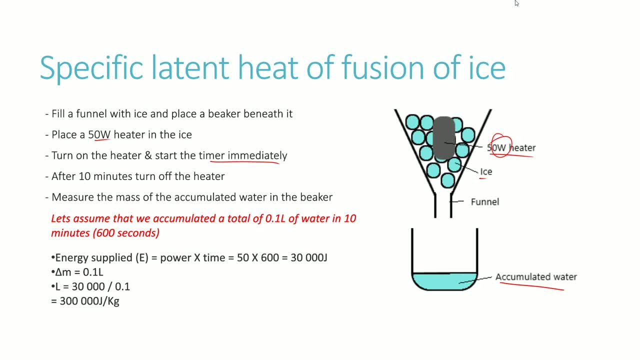 And after the 10 minutes you turn the heater off. So what you want to do is measure the mass of the accumulated water in the beaker. For the sake of this experiment, we're just going to assume that you weighed it all up on a balance and we're just going to say it was, say, a total of 0.1 litres of water. 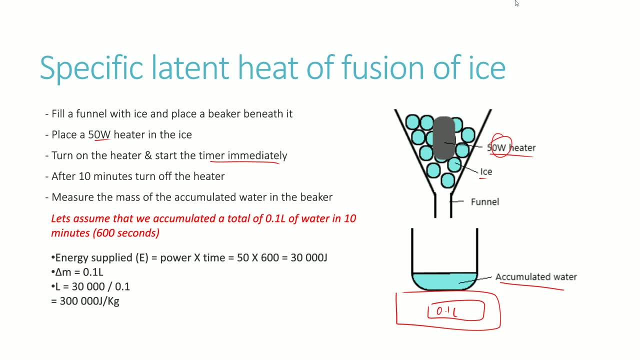 Okay, Or let's just say, 0.1 kgs of water on a balance, and it took 10 minutes, because that's when we stopped the timer, which is 600 seconds. So that's the basis of that experiment. So then, what you're going to do is you're going to sort of go energy, how much energy? 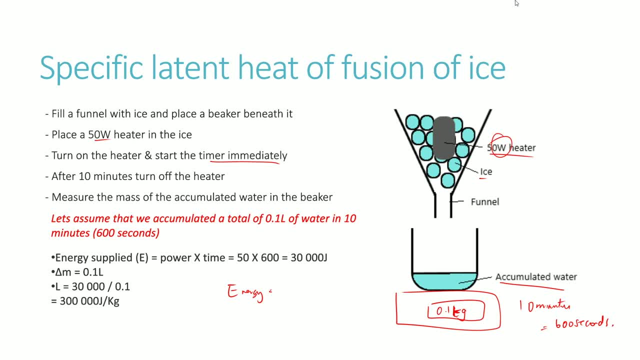 we input into this beaker And then you're going to multiply that by 600 and that's going to give you 30,000 joules of energy that we supplied into the system. The change in mass is going to be 0.1 kgs. 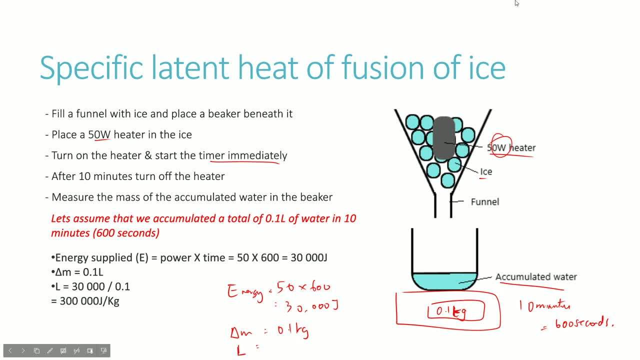 And the specific latent heat of fusion is going to be the energy divided by the mass, Which will result in 0.1 kgs. So that's going to be 300,000 joules per kg. So the formula for specific latent heat of fusion is the energy divided by the change. 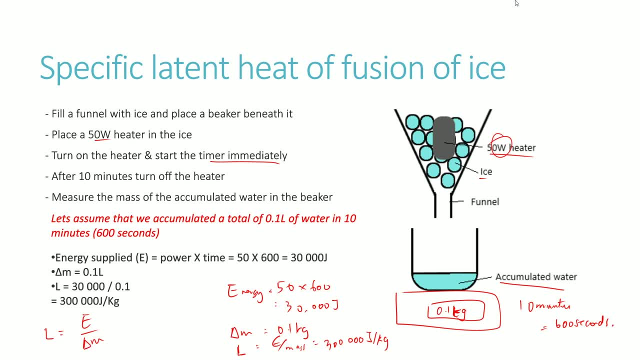 in mass. Which makes sense because if you think about the actual definition of the specific latent heat of fusion, it's again: how much energy per kg are you using to change the energy? So the best way to write that down is to write that down as being the average of geological 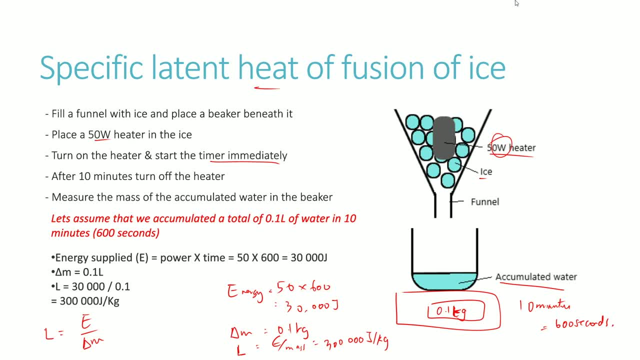 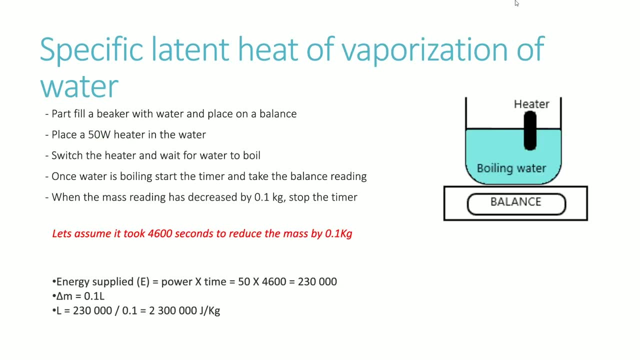 energy And once again, the formula is the energy divided by the change in mass to melt something, and in this case we're using ice. okay, and you can apply the same concept to the specific latent heat of vaporization. where, again, the specific latent heat of vaporization? 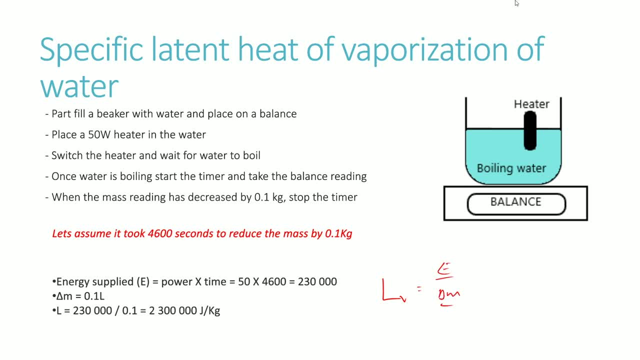 is going to be energy divided by the change in mass, right, and so we're going to carry out this experiment where you put a beaker filled with water and you place it on a balance test to check the change in mass. so you're going to place the 50 watt heater inside the water and then you're 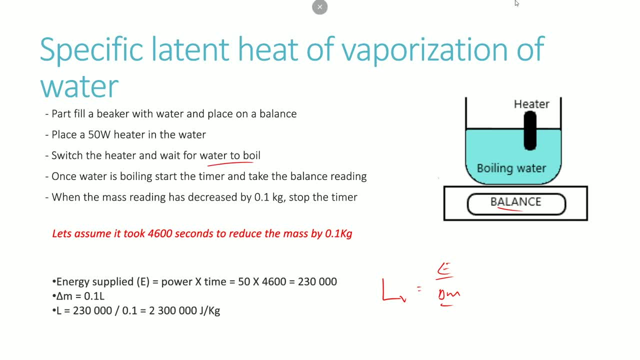 going to start to switch on the heater and you're going to wait for the water to boil. as soon as the water starts boiling, you know it's hitting boiling point, so you're going to start the timer at that particular point. when the water boils, you start the timer, and so you're gonna wait for the water. 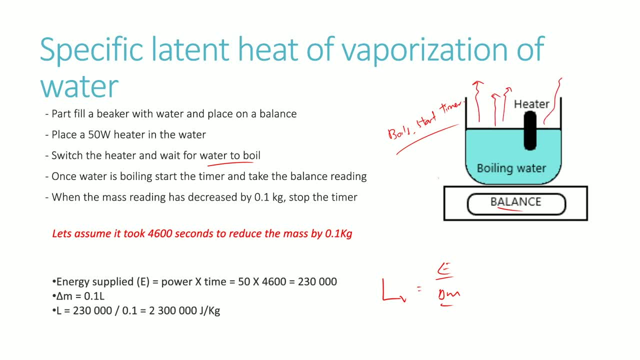 to start to evaporate. you're gonna wait for the water to start to evaporate. you're gonna wait for the water to start to evaporate. boil off, sorry, because we're talking about boiling. the water is going to boil and liquid is going to leave this, the beaker as a result of boiling, and so 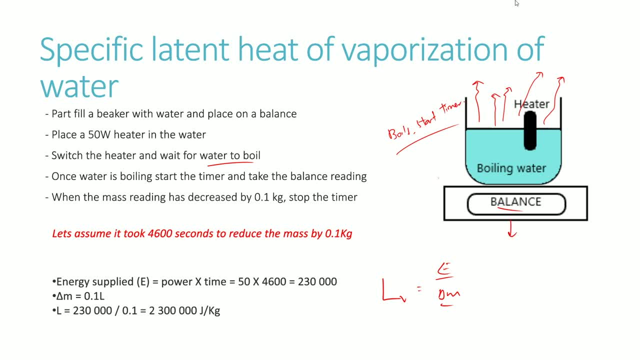 eventually, what that will do is it's going to start to lower the mass of the water as the liquid starts to vaporize. so the when the reading has gone down by 0.1 kg. so if you started off with this, I say you know 0.5 kg when it's gone down. 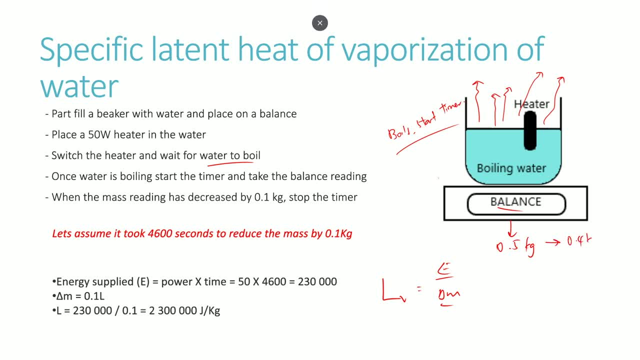 to 0.4, then you stop the timer. okay, when you find a change in mass of 0.1 kg, then you stop the timer. and so let's just imagine that it took four thousand six hundred seconds for the change in mass of 0.1 kgs. well then, you can calculate energy, because energy is power, times, time, right. 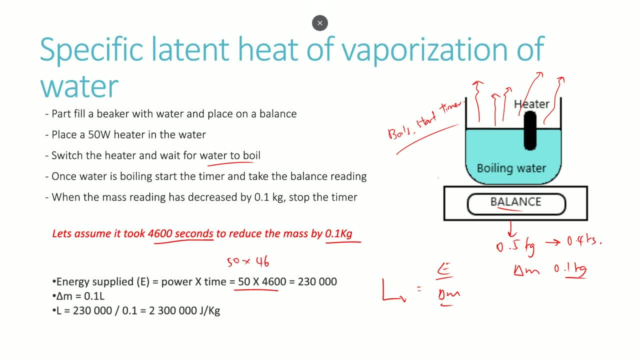 so you've got 50 watt times four thousand six hundred. that's going to give you a value of 20, twenty twentyição, two hundred and thirty thousand jewels of energy. that's been supplied during this time frame and of course, the change in mass is your 0.1 kgs, or. 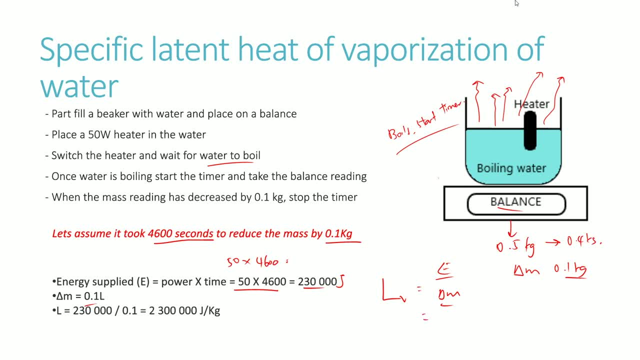 liters. and so when you put that into the calculation of himpedi, divided by the change in math, we've got 23,000. divider by 0.1, that's gonna give you 200 jewels per kg. So that's an experimental setup that you can use to calculate the specific latent heat. 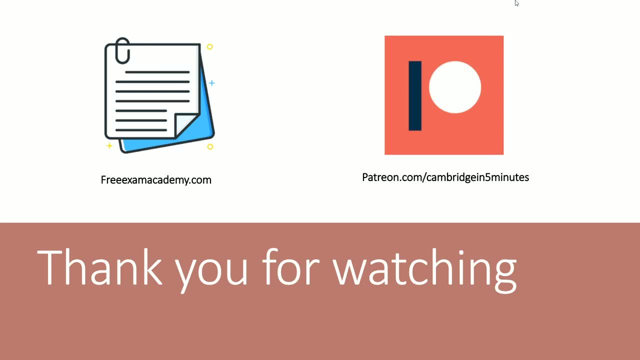 of vaporization. So I hope you found that video useful. guys, For free notes, extensive resources- go to freeexameacademycom. that's my website there. I'm constantly putting new information and things like that on that website For those of you that want extra help with past paper solving and things of that nature. 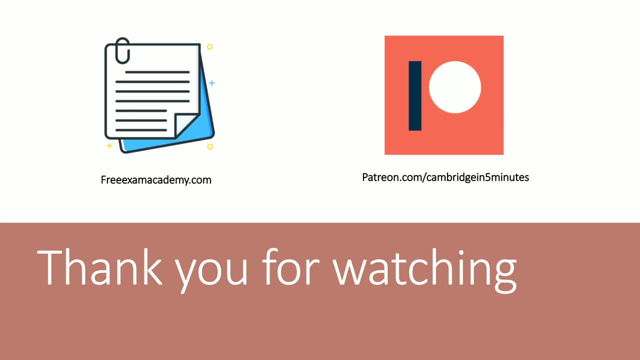 I've got my Patreon channel for a small price of $3 a month. I've got a lot of content on biology and chemistry there at the moment, but for physics I will be putting more stuff on there as soon as I finish the entire course here on YouTube. 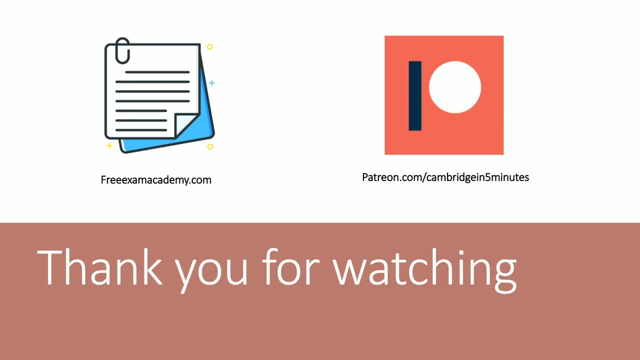 And then the main things will be just going through past paper questions, but I've already got a lot of topic-based MCQ questions there for you to have a look at and some other resources of resources, So feel free to have a look at that. 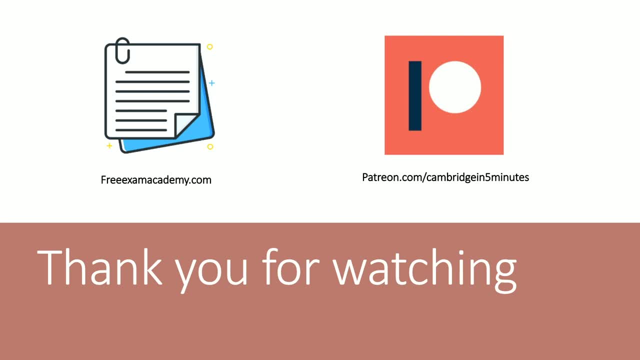 But without further ado, thanks for watching. I'll see you next time, I'll see you in the next.